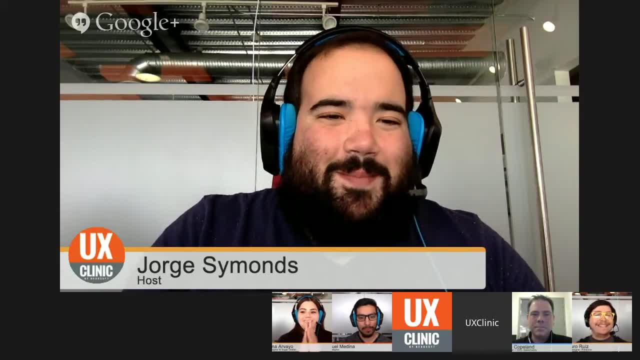 Arturo, do you know the UX Connect? Yes, I want to be part of it, So we're letting him be here today. He's been of great help. His name is Arturo Ruiz. He's also a really talented Pokemon trainer. Welcome back, Arturo. 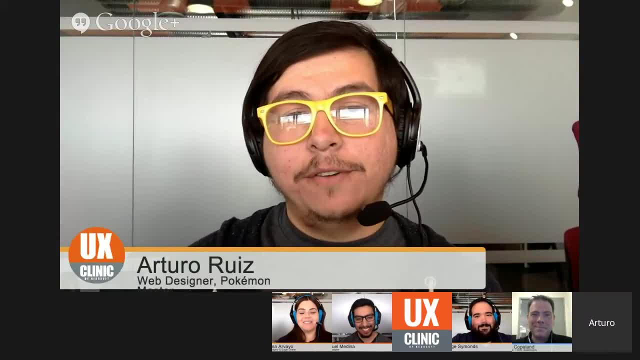 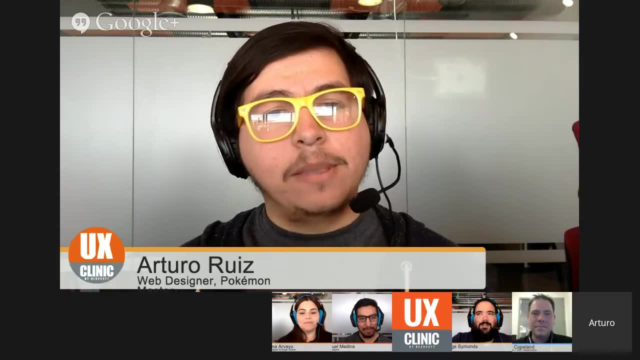 Hi guys, I'm pretty excited to be here. This is my first episode and I'm always been a closet fan of the UX Connect, so I'm very glad to be part of the team right now. So now you're part of the team. No more closets. And last but definitely not least, 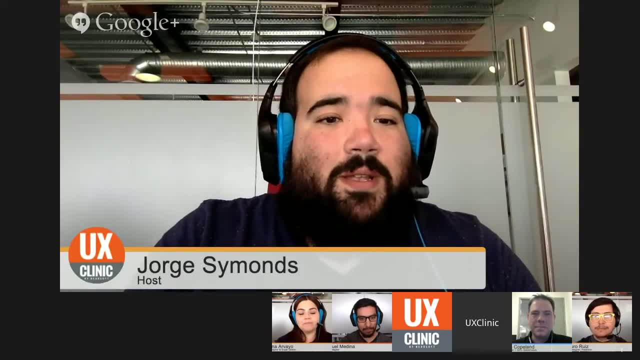 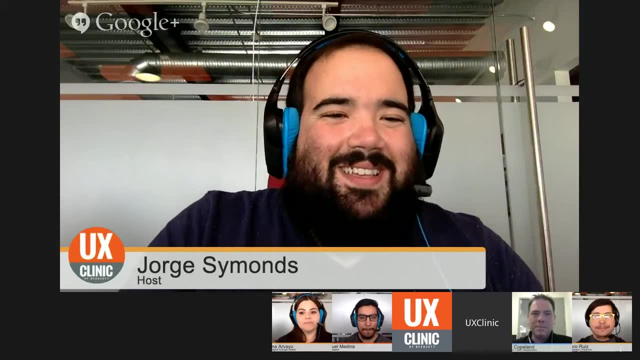 one of the most important parts of our show today is John Copeland. He's the CEO and founder of Sales Caddy, and we're going to give the mics to you, figuratively speaking, So you can tell us a bit about your role and what Sales Caddy does for. 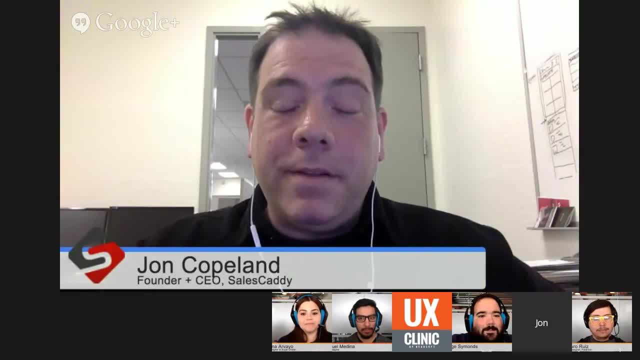 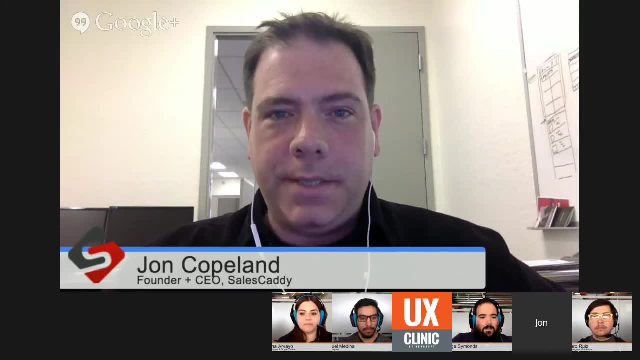 the, for the, for the, for your users. Sure, Thanks everybody, and thanks for joining us this morning. I'm really excited to get some good advice about UX. So Sales Caddy is an iPad based sales enablement tool that gives reps more time to sell. 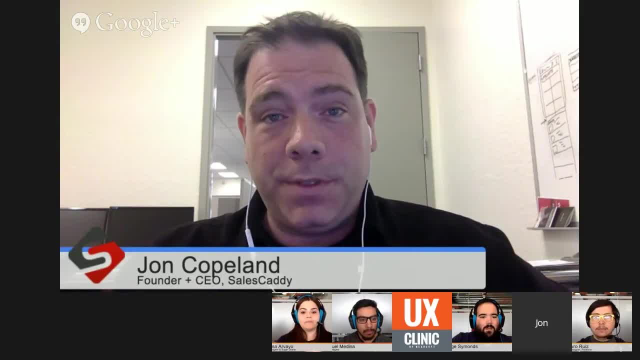 and all the answers that they need when they need them the most. My job here, obviously, as founder. I lead product promotion and business development, and I have a team of developers who are ready and waiting to put some of these recommendations into action. Well, that'll be. 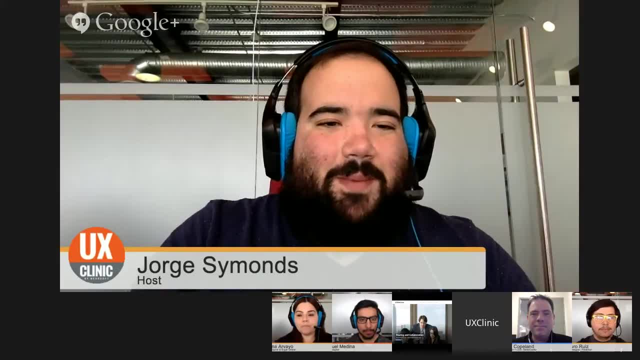 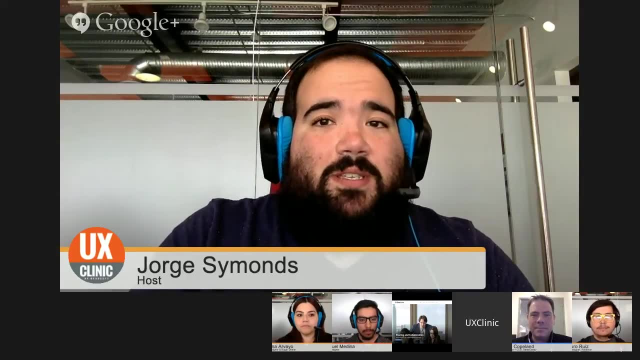 great, We can ask you to stay hang with us for the next 10 to 15 minutes and you can see a lot of interesting information. So let's kick it off with asking the our traditional question, which is: why did you guys choose this particular design method called heuristic evaluation for Sales Caddy? 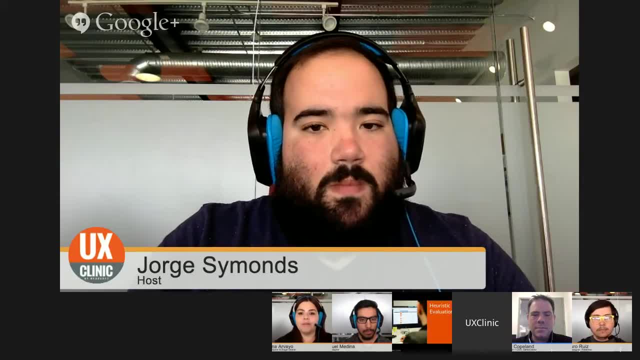 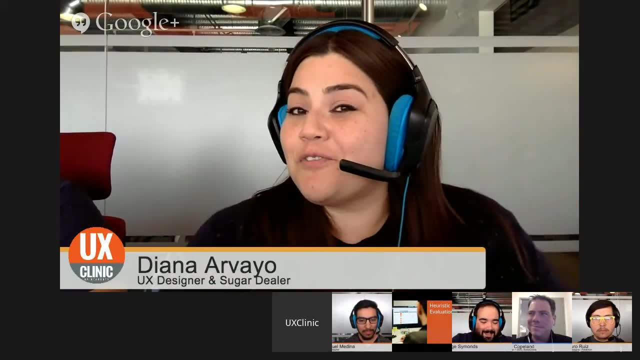 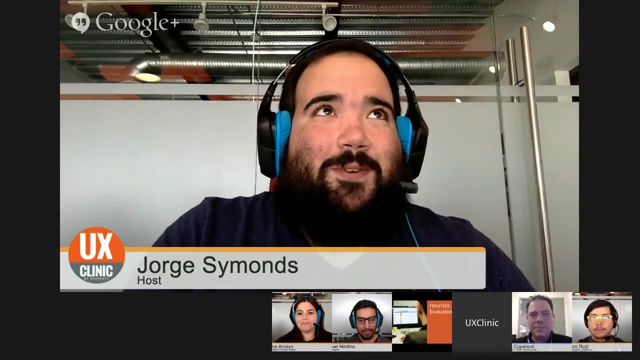 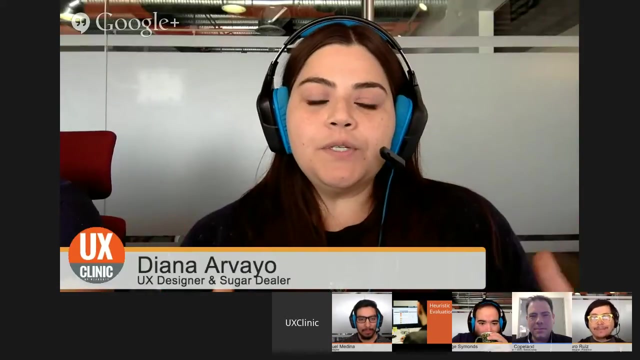 Yeah, we choose heuristic evaluation, and I thought you will be more enthusiastic and dramatic when you pronounce heuristic because I thought one of your favorite methods episode I was in heuristic evaluation back in like 2014,, so I'm gonna do it excitingly next time, I promise. Yeah, okay, thank you. Well, we choose heuristic. 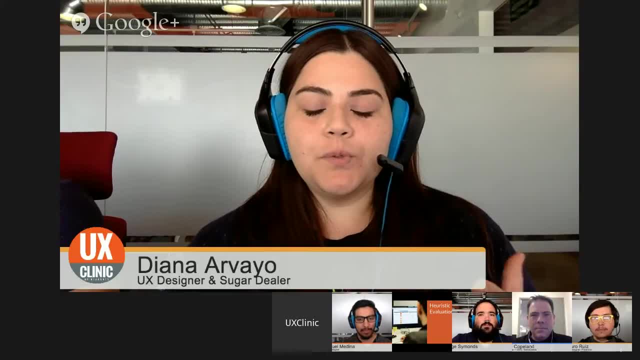 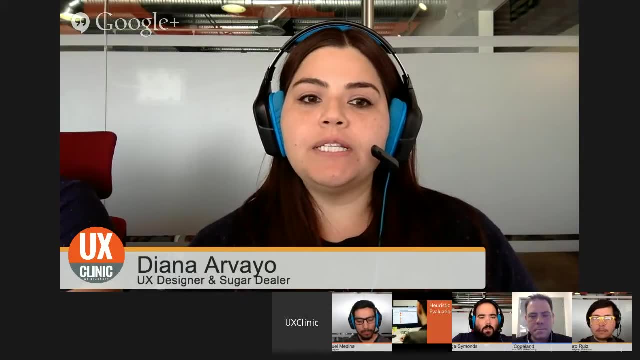 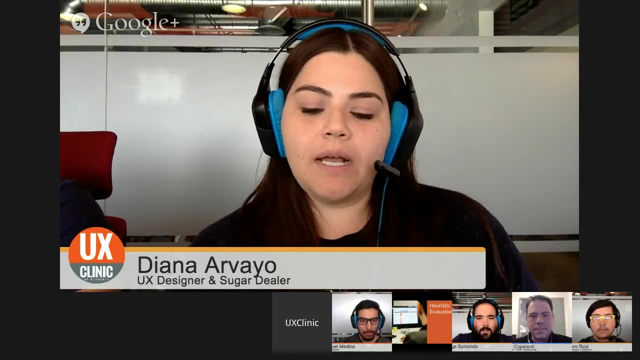 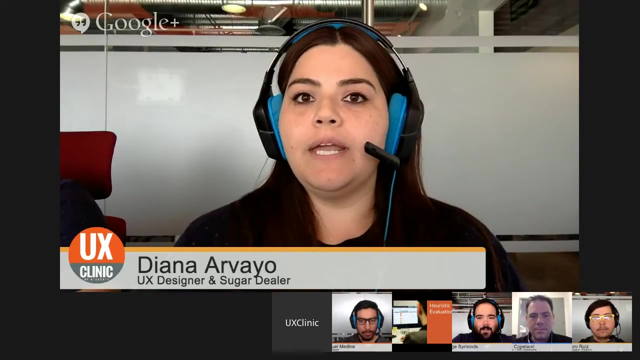 evaluation because, first of all, it helps to identify usability problems in the user interface and also it helps you to detect and reduce the number and severity of design errors. So when we started our research as a team, we decide to look for a method that will help us to evaluate and identify usability. 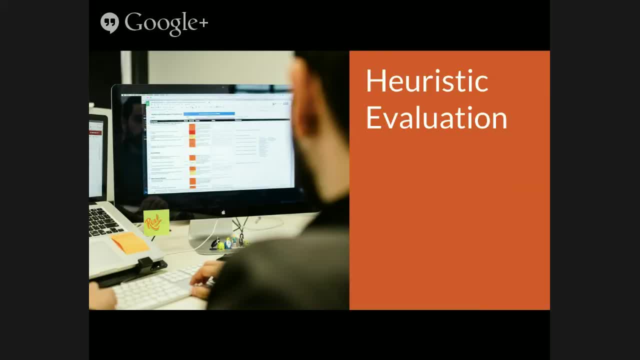 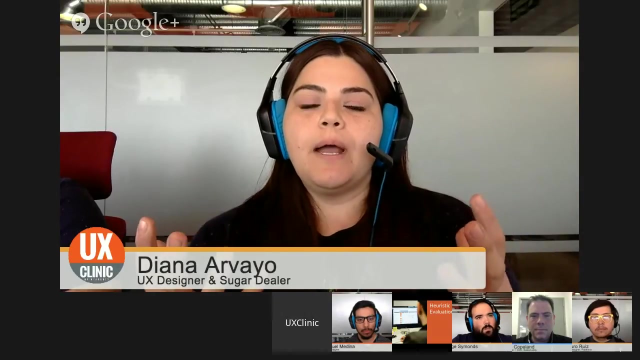 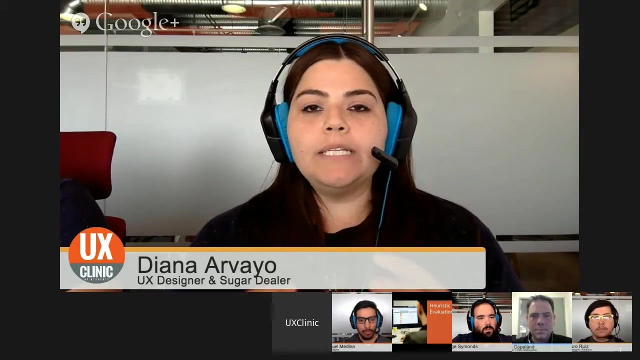 problems. And heuristic evaluation is great because it follows the ten principles of usability. so we decide that it will be the one method to do a research. But also we choose this method because it provides a global panorama about the weaknesses and the strengths of the system. So we did the evaluation. So you have. 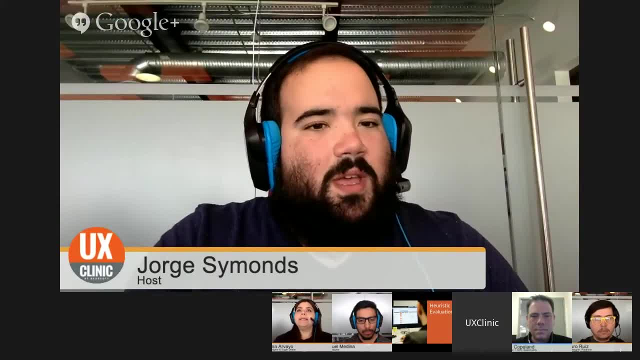 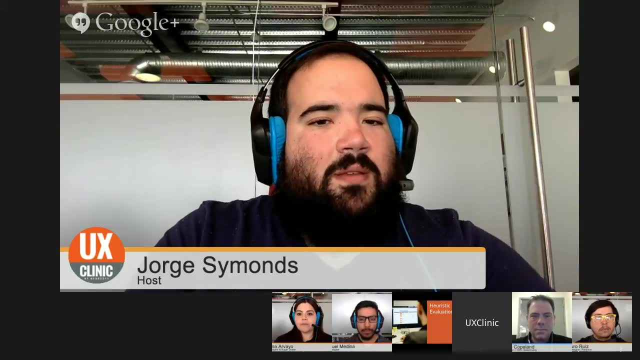 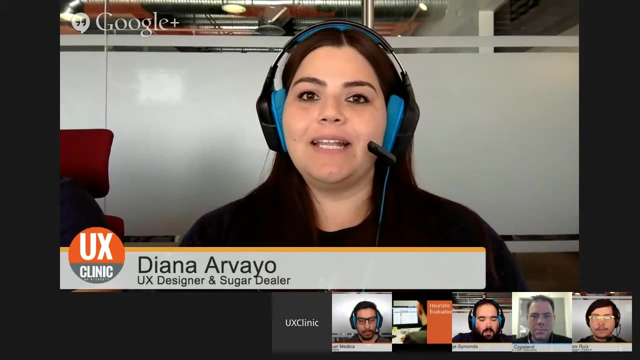 like ten preset UX principles and you compare and contrast that to the user interface of Salesedu and that's all. You actually went outside, you thought outside the box and started talking to users to see if that information was correct. right, Yeah, that was. I want to say that We also interview different real users only. 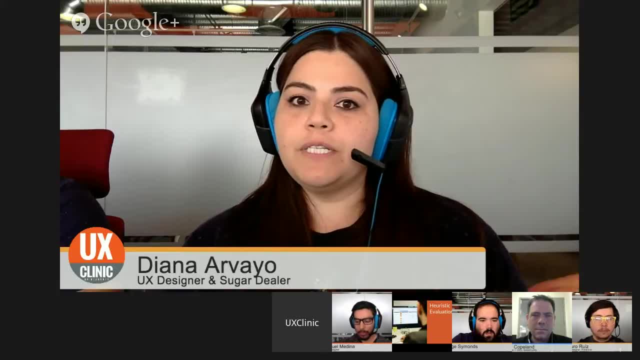 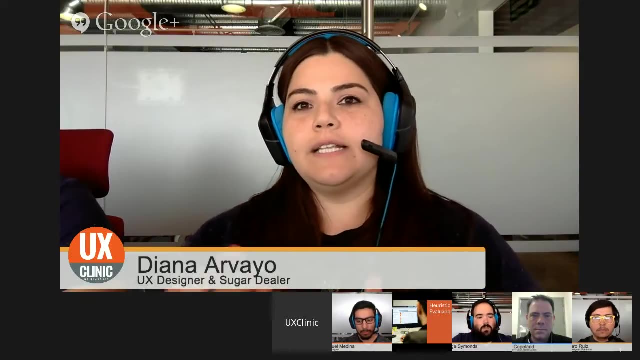 with the purpose to see if our findings from the heuristic matches with their feelings, and the answer is yes, A lot of the things that we found from the heuristics matches perfectly with the feelings of the users. The things that they delight most and the things that they make them frustrated matches perfectly. So today we 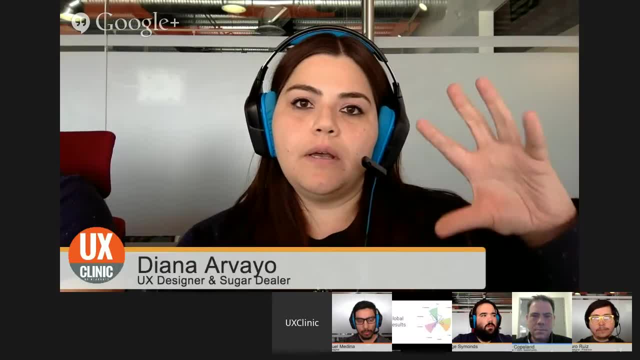 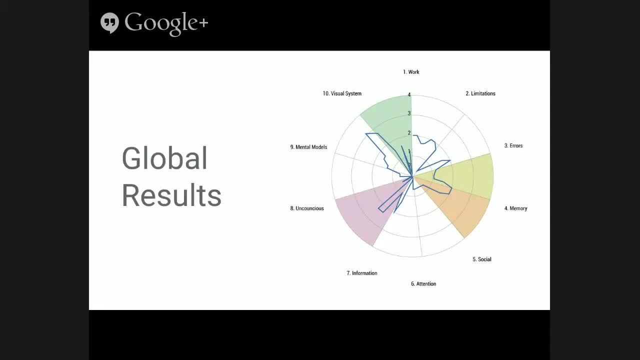 are going to present first of all global results Here in the chart. maybe it's a little, I don't know, technical or it's not super visual attractive, but we are going to move quickly from this chart to see the improvements that we are suggesting. So here we have the ten principles that I already 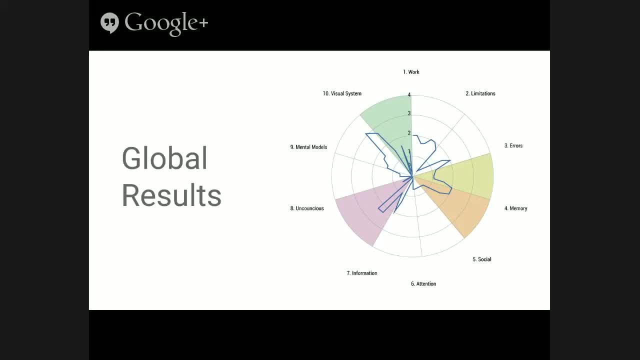 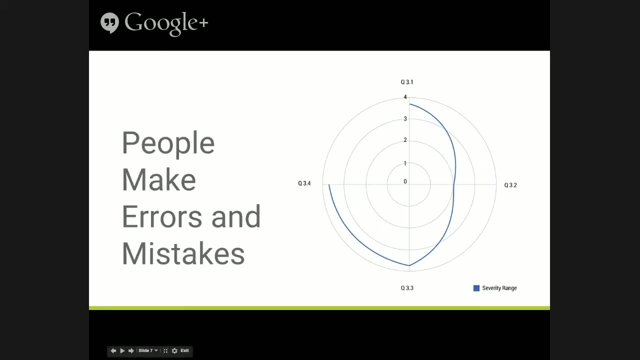 explained and we have the four main opportunity areas for self-guiding in these ten principles. We have the errors, the memory, the information and the visual system. So let's move to each of these different principles with feedback. So who wants to start? I think I'll start. The first one is people make. 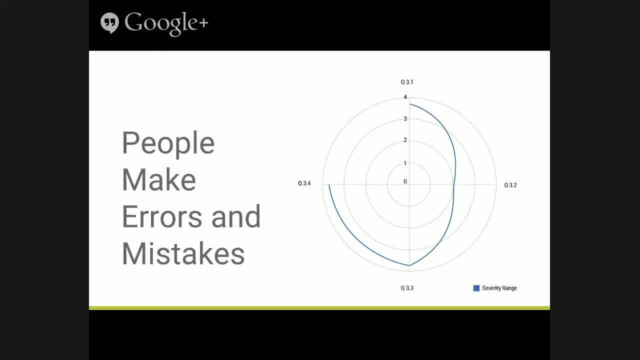 errors and mistakes. So we can see in the chart that we have four of three questions that went highly with critical feedback from the heuristic and the severity range is kind of high. So the reason of this is the console is not prepared for errors or not, that it prevents the user when 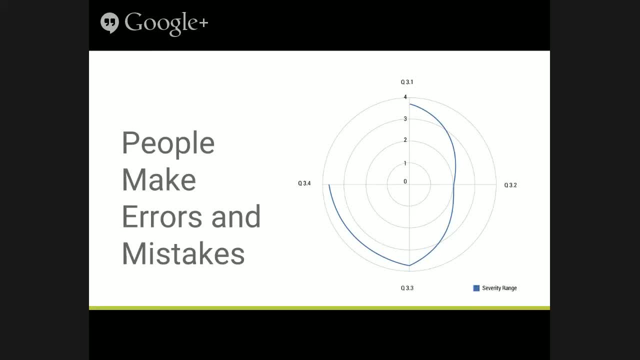 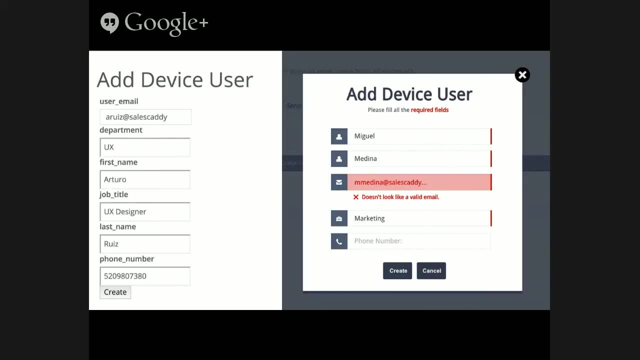 they're having a mistake. So I'm going. I would like to show you guys some some examples We have. we we kind of have a user model, So here we can see the fields in which users can type all kind of information and the system validates. 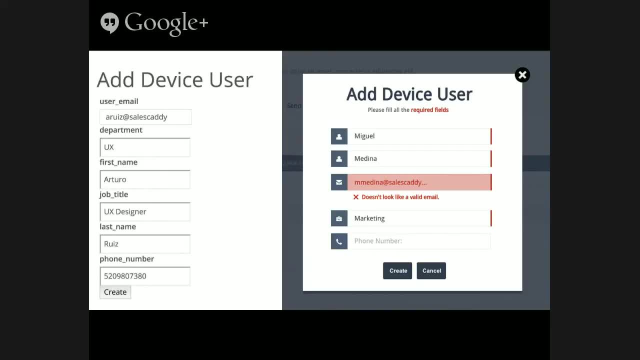 that information So you can. you can write whatever you want and it will create that user, even though that's not valid information. So what we want to do- improve here- is to have a kind of a feedback letting the user know where they are making the mistake while typing that information, so in the right panel. 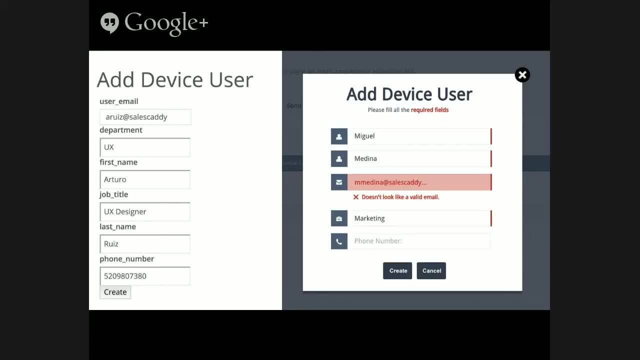 we have an example: an email is a typed wrong, so the the console gives them feedback that that's not a valid email, so please try it again, and then allows the user to create that that user, instead of just creating the user with the wrong information. so and this is a way to prevent the error, right, yep? 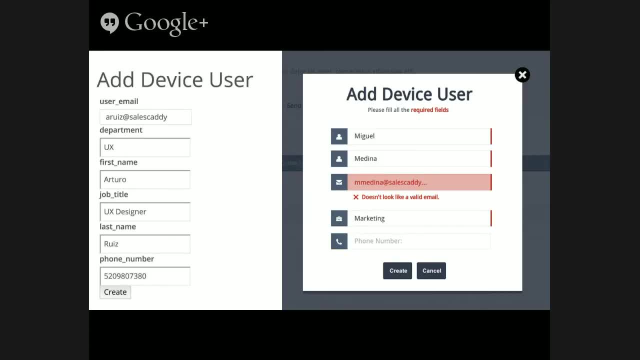 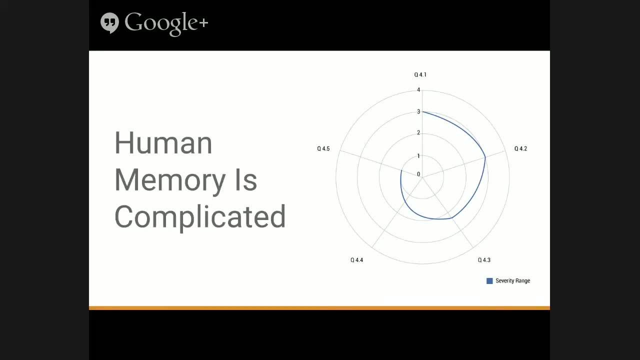 exactly that's what we tried to do. and the second one is: human memory is complicated, so at first we have a lot of information displayed at once, so the user have trouble finding what they want. so what we do is we have a lot of information displayed at once, so the user have trouble finding what they want. so what? 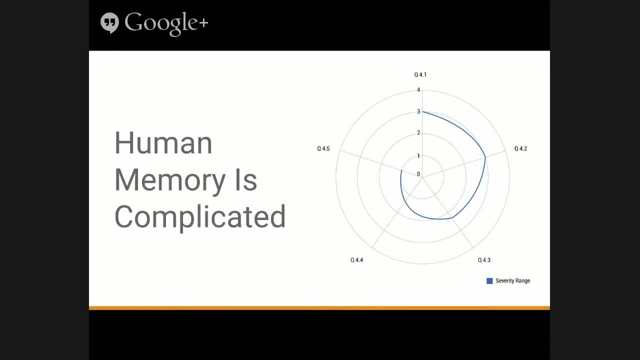 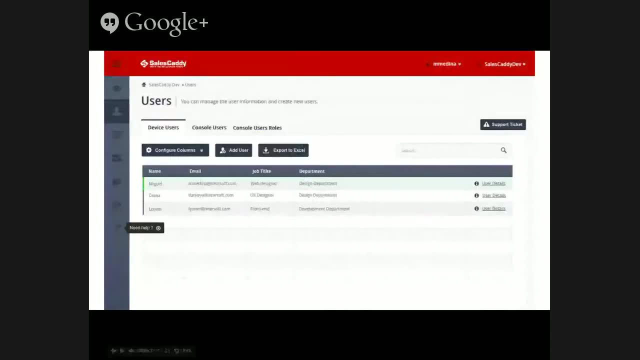 we are proposing and we want to show here in the mock is I: we want to group all the related information, for instance, device users, all related to device user will be there, all the tasks, and this will prevent the user to cut the tax flow they are having. so if they want to create a user concerning device user, 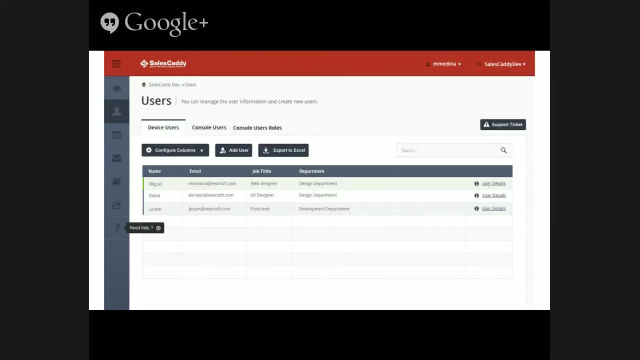 that's when they're going to find the information and if they're, they want to know something about console users. all that kind of actions will be there and they won't have to search for them or remember where they are. so all are creating in groups, so I was. I was gonna say it's. it's about not trusting the. 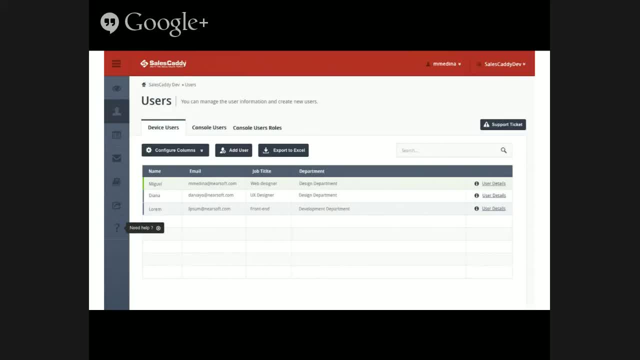 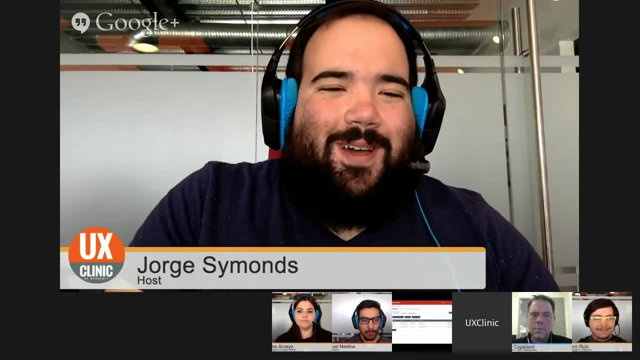 user, but I think it's the other way around. it's simplifying the way around the user so they don't have to worry if they- I don't know- misspell their name or who would misspell their name. right, wait, but I write their email incorrect. 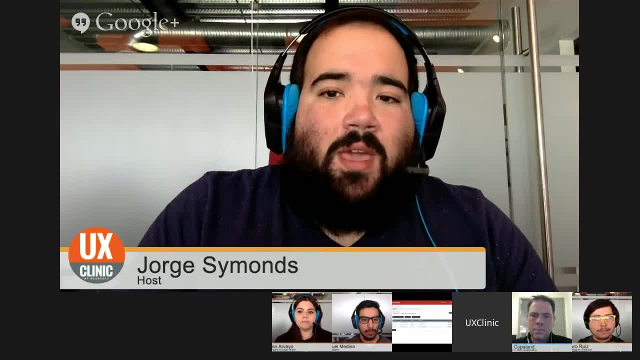 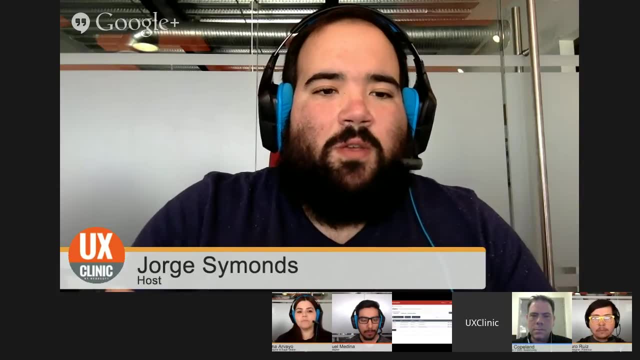 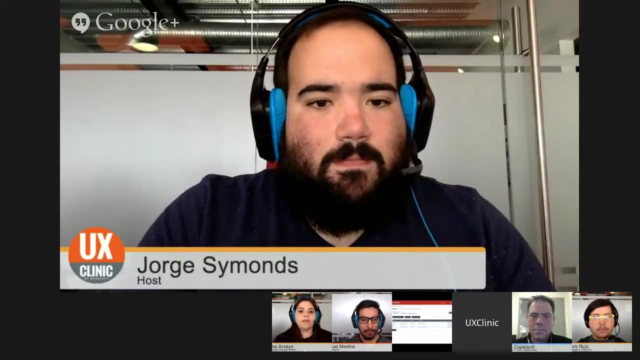 so the interface would tell them: hey, your email is wrong. and instead of the user having to go away from his regular test flow, they can find all the single user information, for example, in a single place with some visual clues and stuff like that. so, okay, yeah, also, it's a beautiful interface I am very proud of. 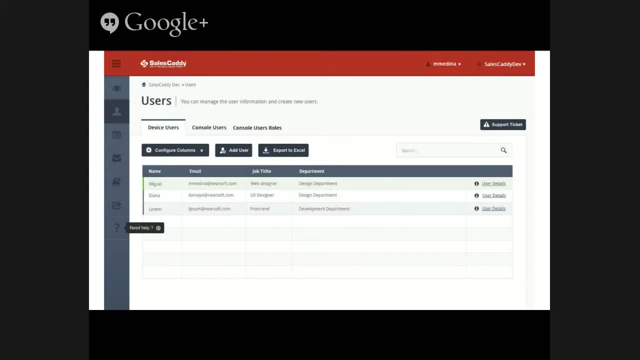 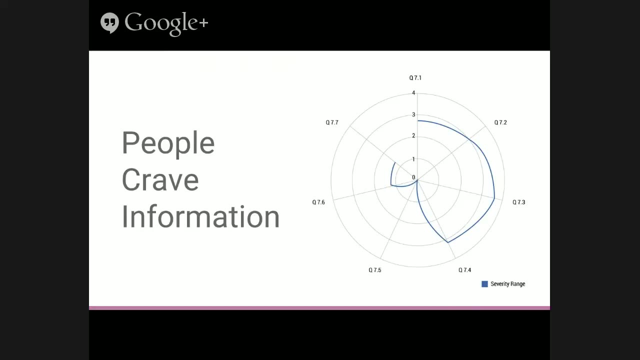 that, because I think this very bright and all the things come pop up, but we're going to explain more about this thing. in short, the theoristic that we found opportunity areas for so, Scotty, is related with the information, and this heuristic is called. people crave information, and here, here's the thing. 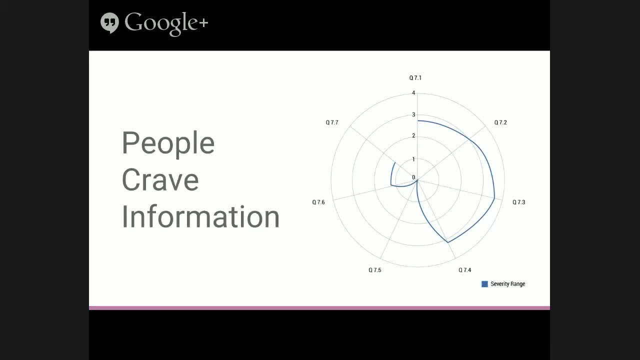 people wants to feel in charge of the things that they are doing. for example, here right now I'm talking with John, with Arturo, Miguel, Jorge, on the people from the audience. so I expect that if I'm talking, see at least a gesture from from Arturo, maybe his head or the hands or or Jorge. so if we having a 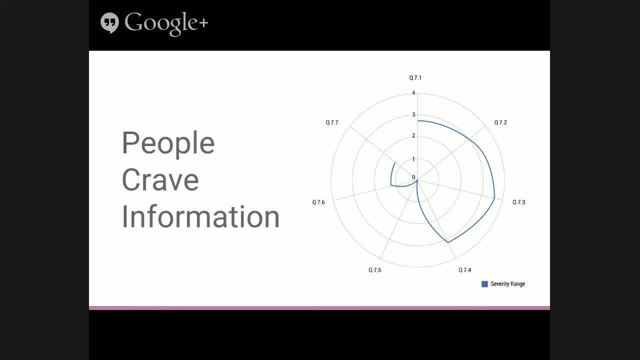 conversation. I want to having the same channel and receive some feedback from you. it happens the same with the system. if an user do an action, he wants to to know that the action is doing and receive some feedback. for example, in the next mock-up we have that when a 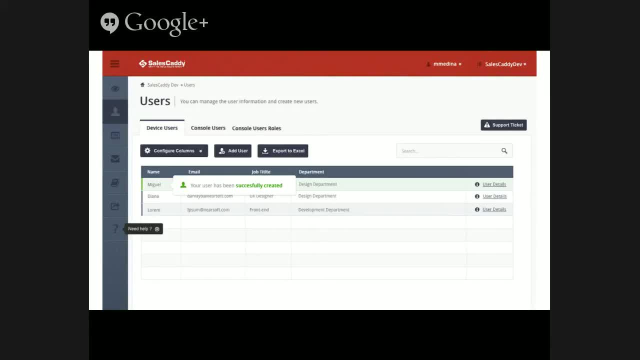 user creates a new user in the console, a little message appears and say: there are you. your user has been successful created. that's the way to let know the user that the things that are he or she is doing in the console it's taking action and it's that way that communicate between the system and the 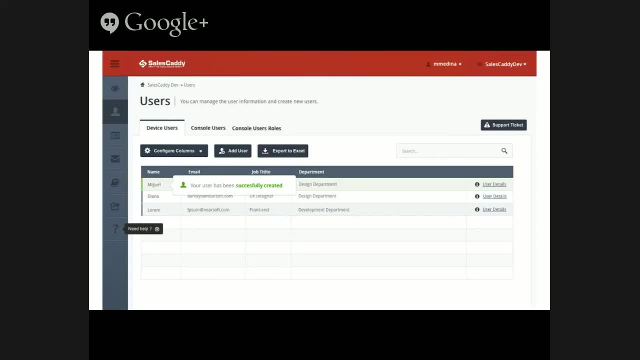 user. also. this heuristic is about to help them when they have problems. for example, we are proposing to add in the left and main menu a section for help. do you need help? there is, and this section will contain the most common questions that the IT department receives every day, so in that way the users can click on it. 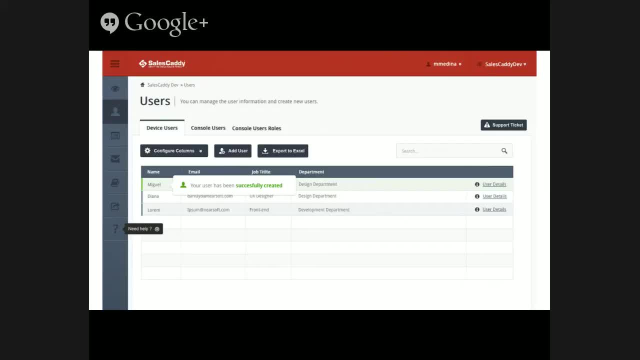 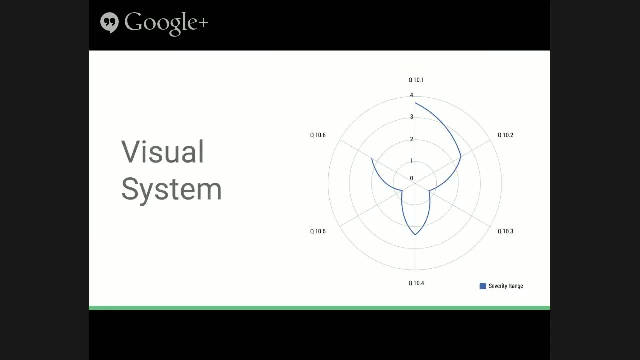 and read the most common questions and have some answers, and that's the way that we are proposing to solve and some of the some of the findings that we got from this heuristic. the last of the opportunity areas that we're discussing is the visual system. this heuristic is all about how the information is displayed around all the 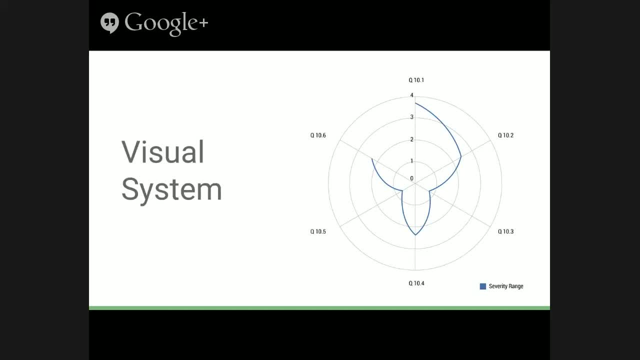 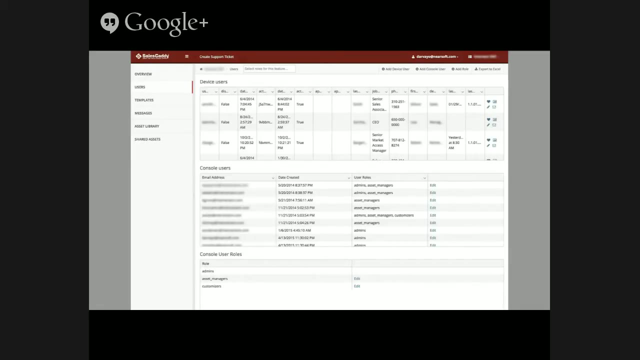 console and how they make use of a graphical language to represent this information. we take three major highlights around this heuristic. the first one is: I can see graphics right now. the console doesn't have any graphics or icons or any way to represent the information they display around. the console is just a. 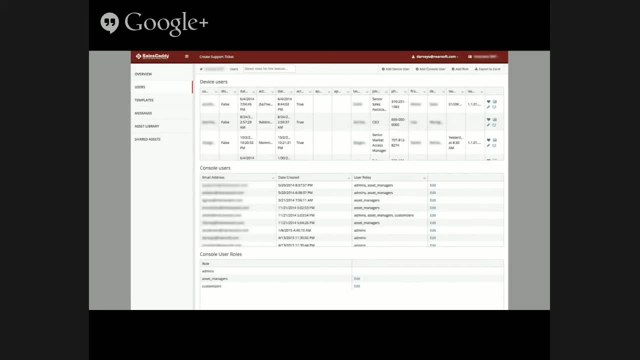 sea of plain text and the only four icons are there on the tables. they're really hard to translating what they actually do, what they actually mean. the next one is hierarchy and color coding. right now, the hierarchy of the information of the console is confusing, making more relevant information to be 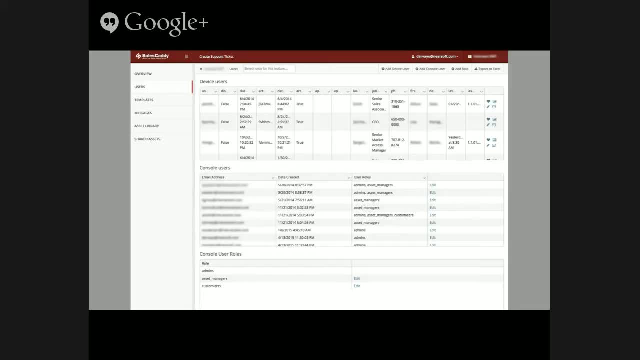 confused with the information that is not so important. grouping similar information helps the user to focus on a single task instead of surfing around the information that is scattered all on all the console. also, the application doesn't take advantage of color system or color coding to represent different status of. 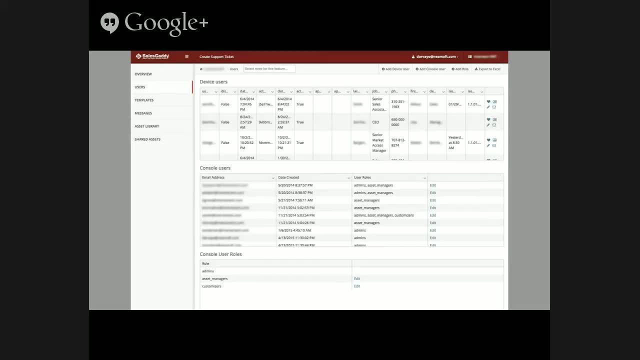 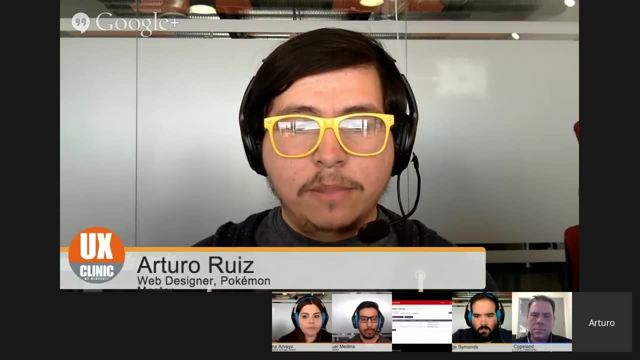 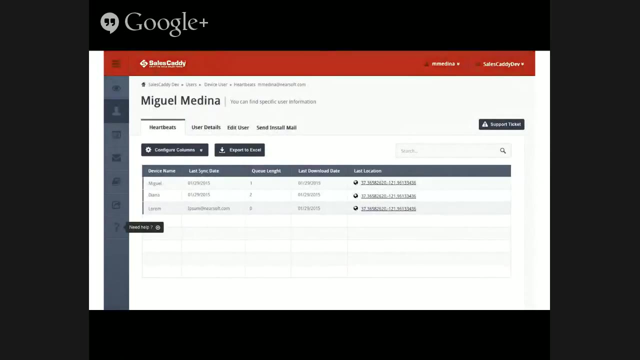 interactions, for example error message or success messages. on the following screenshot we can see the interface consists mostly on plain text and the color coding is actually is not there. and the last one, and here I'm quoting, I think, in a quote of some of the users that we interviewed. it says: 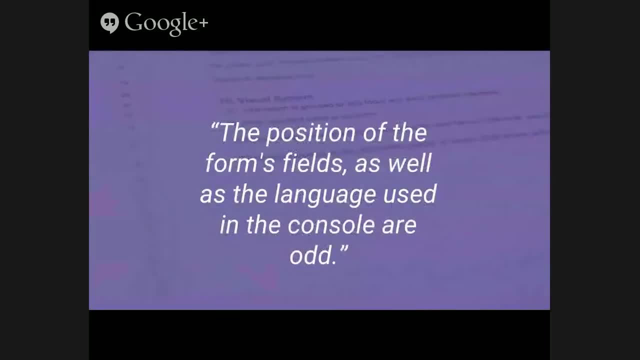 that the position of the form fields as well as the language used in the console are odd. the next point is the technical language. the information displayed right now on the console is in a technical language, is important directly from a database and most of the labels and most of the table of the information of the 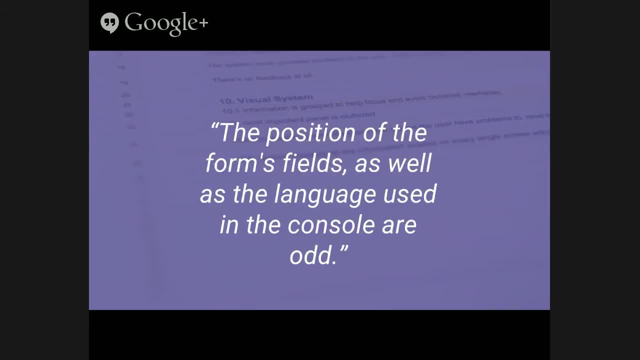 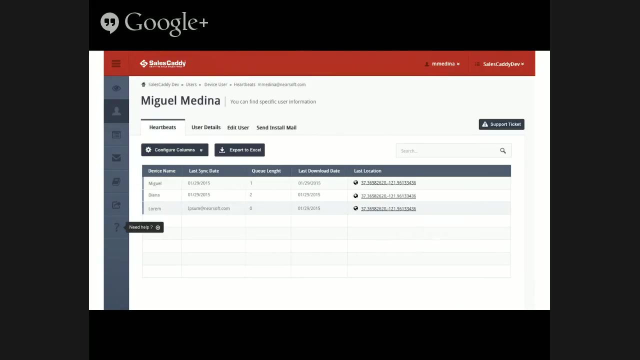 of the tables are in this way, So for us it's pretty difficult to understand what's going on, how to interpret this information. So this way we get confusion for the users because they don't really understand what that information means. so how to work with that. 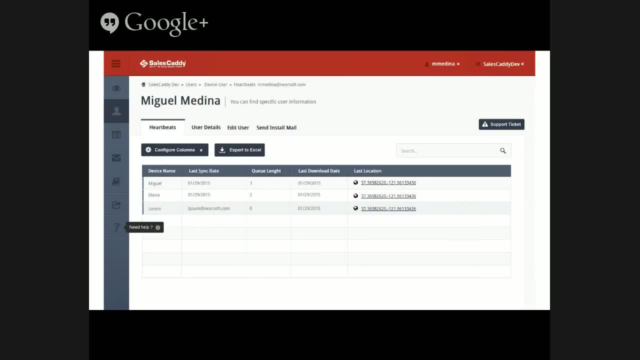 On the next mockup that we see there we can see that we are proposing to make use of some color coding to represent some important inputs on the interface, For example the configure columns buttons or even the support ticket. that is actually kind of missing on the actual console. 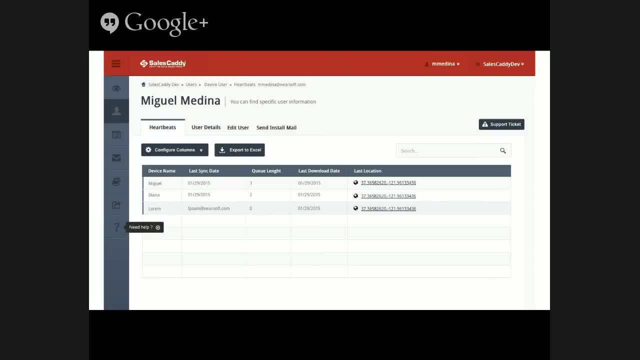 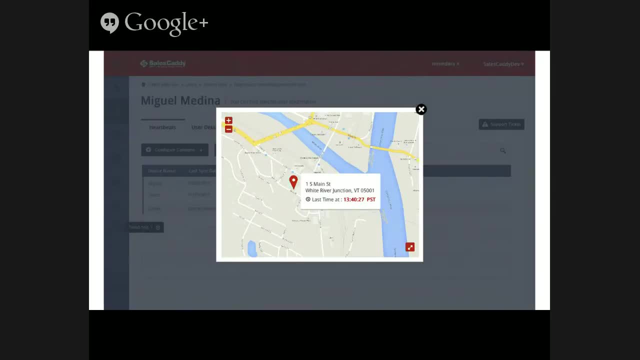 And, as I said before, there are areas where the application can take advantage of a graphical system. For example, right now the application displays the local code. The application has a set of coordinates which most of the users can understand. Come on, who at this work can really understand coordinates? 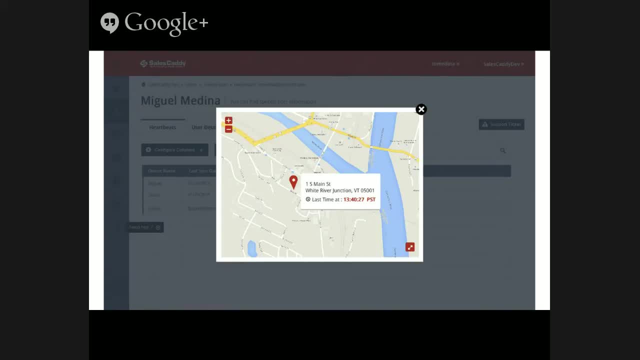 Even Boy Scouts has a hard time interpreting this kind of stuff, So we're proposing the use of a graphical system for this, like a map. A map is something that most of the users can understand and they can easily translate this to something useful. 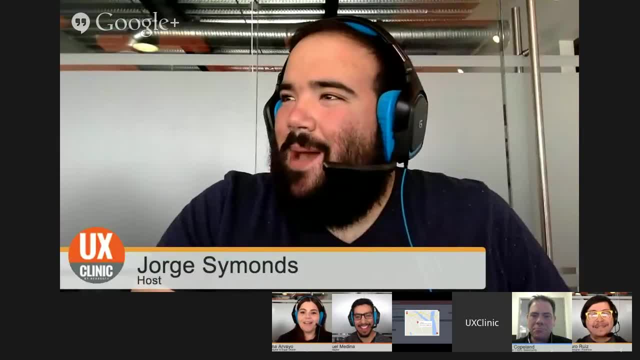 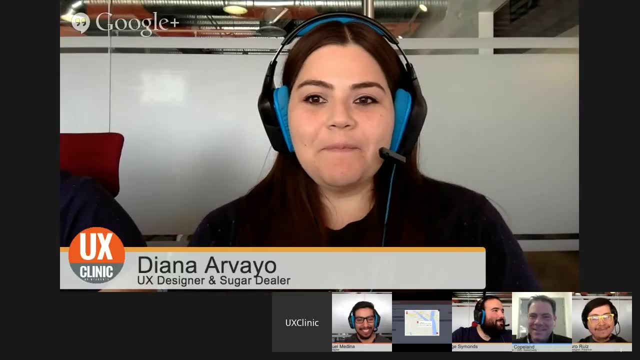 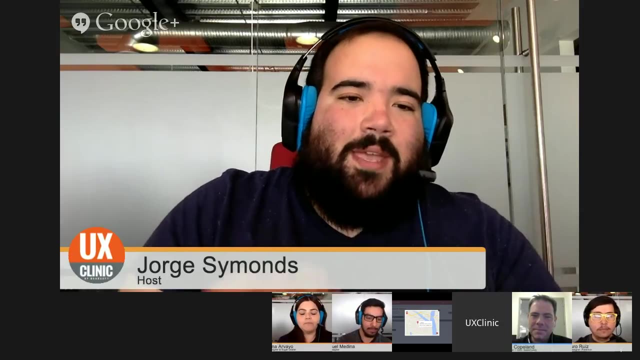 I can understand maps, though I need maybe coordinates and then a map and then a. I have a map. I have a friend that maybe knows how to translate the coordinates. I think We need classes from your friend, So it seems like it's in a way guiding the user through feedback in every step of the 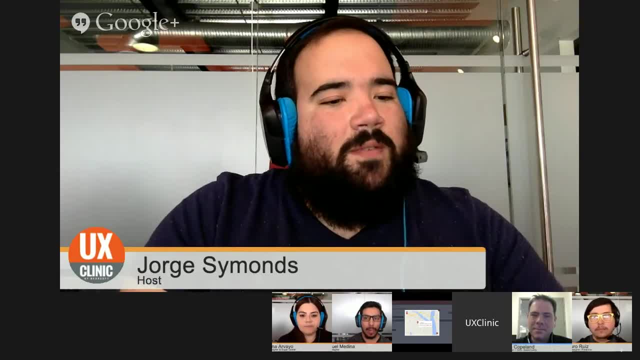 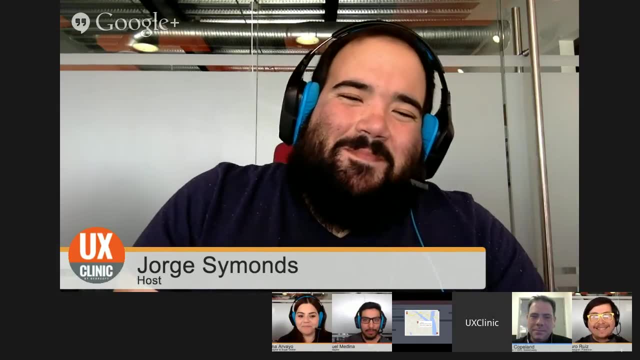 way, having it color coded so they can know what's more relevant to them and what's not. And again, not trusting the user kidding. So in a way, anyway, this is my favorite part of the show because, after all the information, 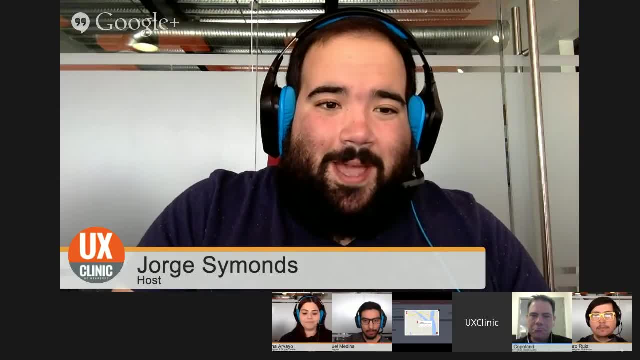 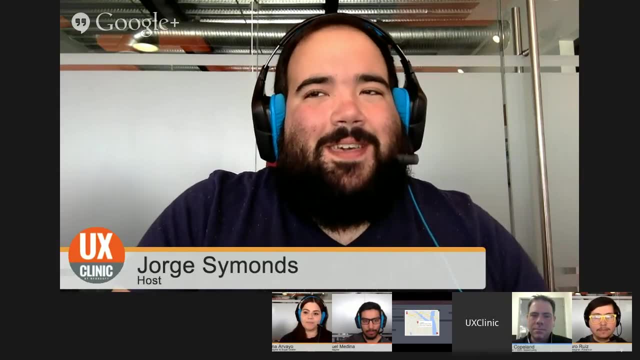 because we're making it hard on John, because we're getting his feedback. now we have four takeaways before we go to ask questions to you. So just in the issue of fairness, we're going to try to summarize it up again in four small 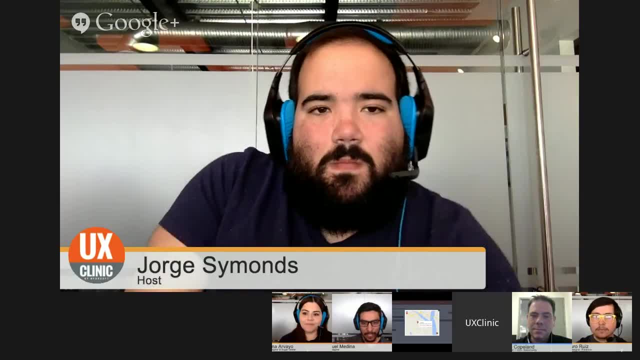 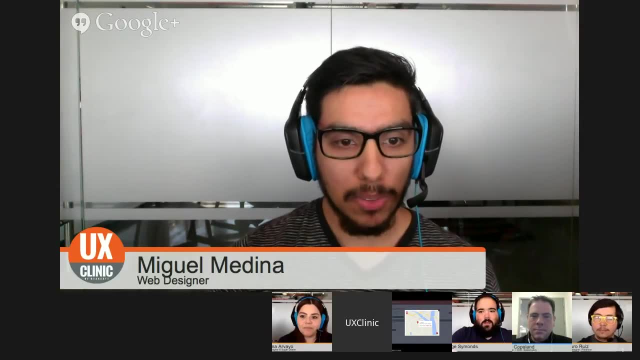 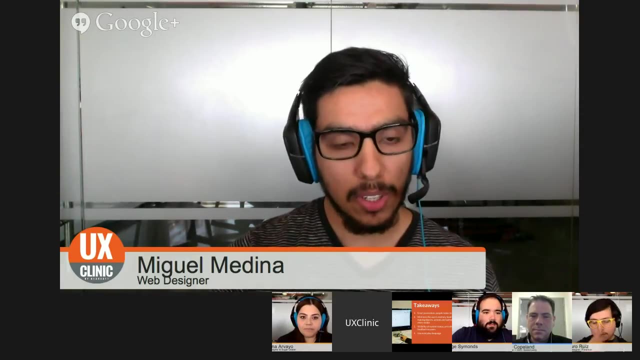 takeaways. So go ahead, guys. So the first one is error prevention, and people make mistakes. So, as I was explaining before, what we're trying to do here is to prevent the user or give them the means to correct that mistake that they're having at the time. but mainly, 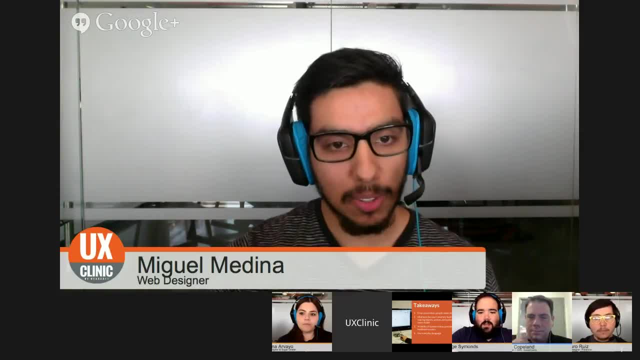 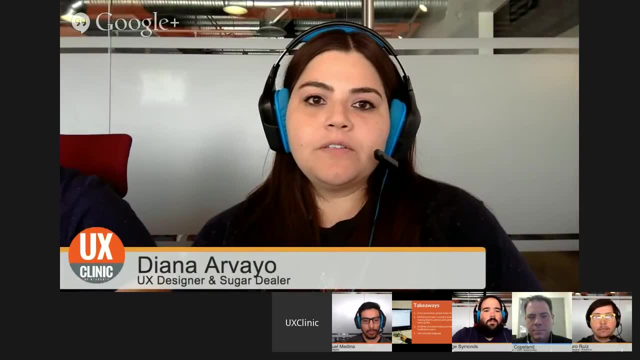 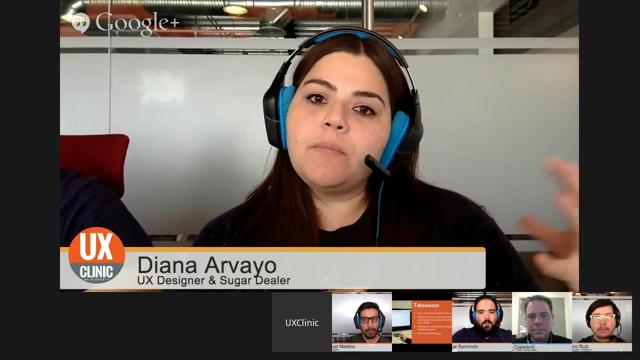 to prevent it. So we want to have that on this console. Yeah, and you can help them with small pieces of feedback and you can prevent a lot of mistakes. The second takeaway: it's about minimize the user memory load by making the objects actions. 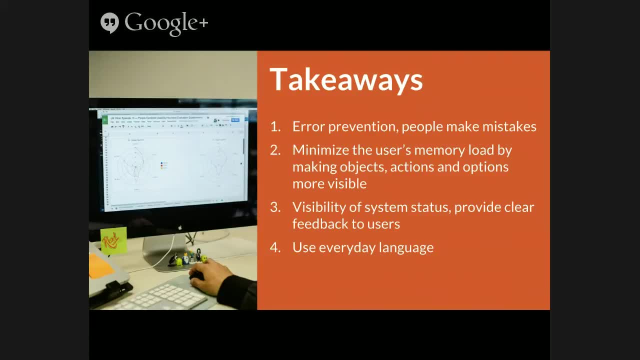 and options more visible, And this is about that. It's all about how you organize the information as we see it in the mockups. we are proposing to have all the information related with device users in a single tab, with their own buttons in the same place. 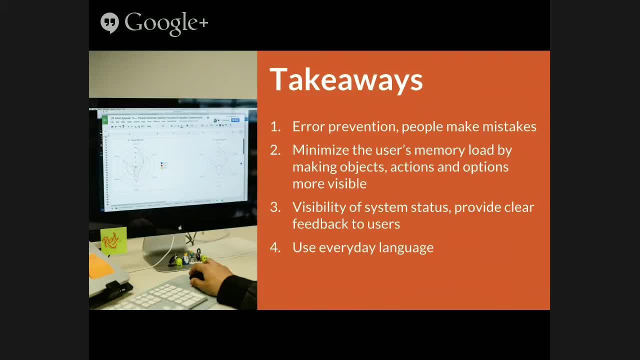 So this is also about use the color in our favor, in our advantage, and make these icons and these graphs come more pop up. The third takeaway. The third takeaway is about the visibility of system status. Provide clear feedback to users, And this is about the. I already explained it. if I'm talking to you guys today, I want: 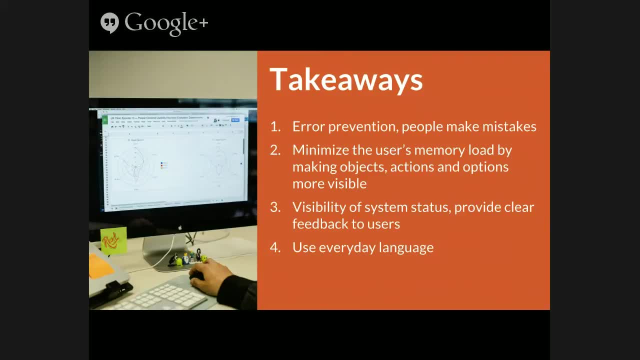 to see your faces, I want to see your eyes, your mouths, your arms. it's the same with the system. The user wants to know what is happening and, if their actions, it's in some way to communicate it with the system by feedback management. 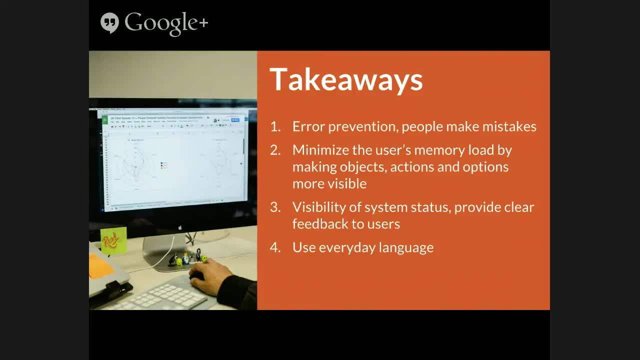 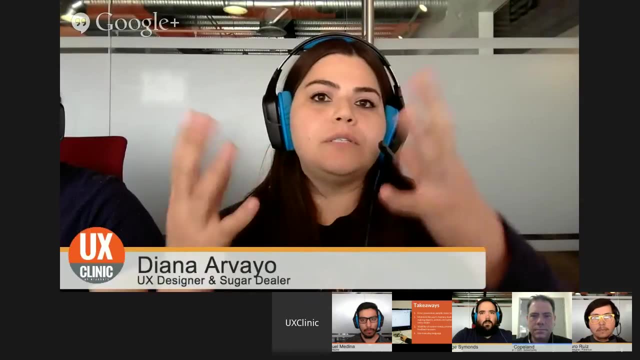 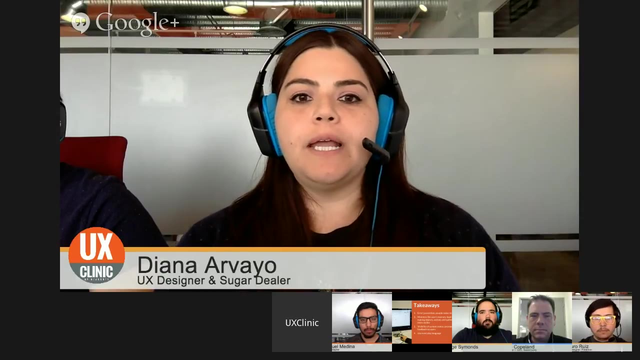 Yeah, And this feedback messages and this feedback messages it could be in different ways, with color, with side phones, with small icons, and I don't know some translations. So this is super important and it's crucial to make the users feel connected and build. 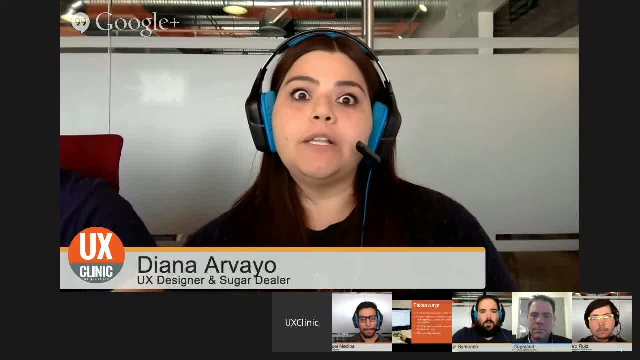 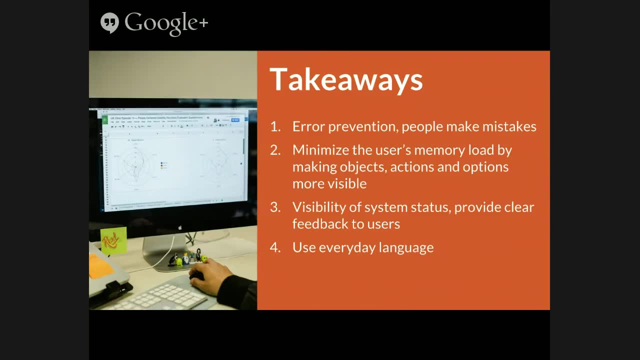 a trust channel with the system and the user. And the last one is: Use everyday language. We're not robots yet, so technical language is pretty difficult for us to understand. Using an everyday language is the best way for the users to understand what's going on. 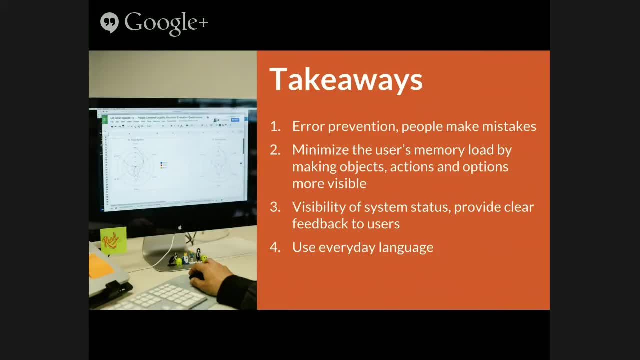 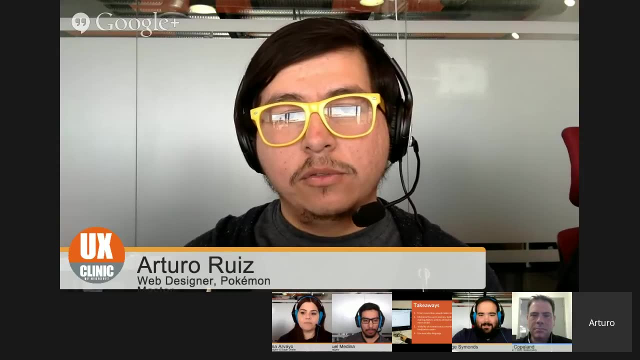 around the application or even how to use the application. For example, the recycle bin on our computer resembles a real life trash can, which is the place that you put the things that you don't need or you have to dispel. So using that kind of metaphors around the application makes the user feel more familiar. 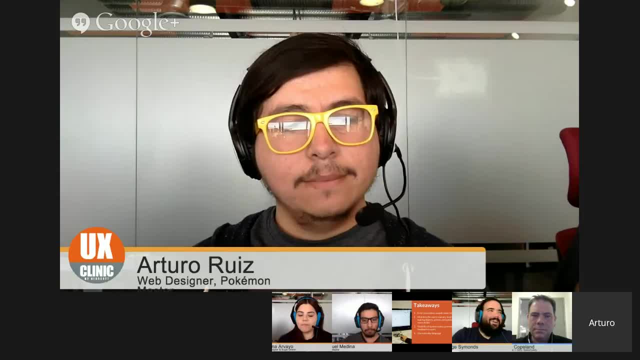 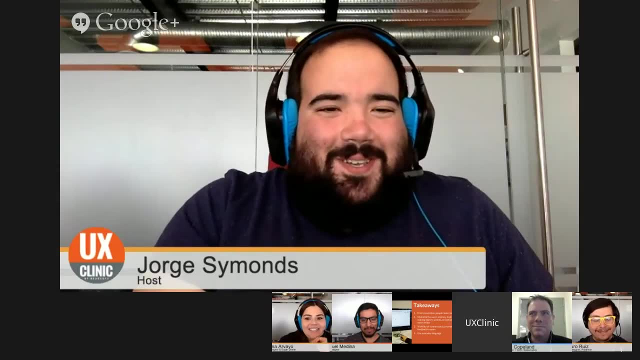 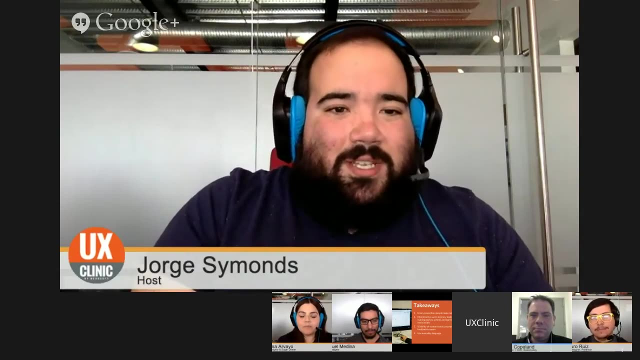 with what they're doing. Okay, I just. Arturo's comments are like the greatest, like he has hope for the future when we're all robots. but okay, So now let's go back to John. I know it's a lot of information, but do you have any feedback? we could use questions. 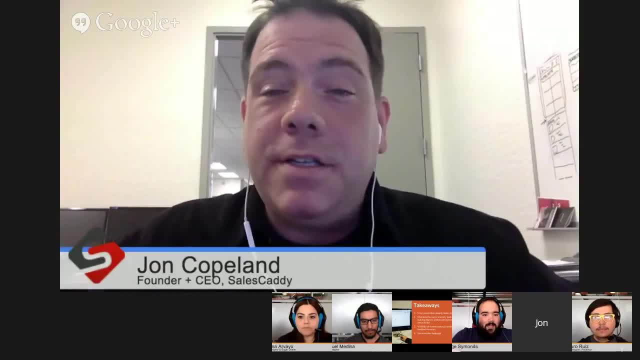 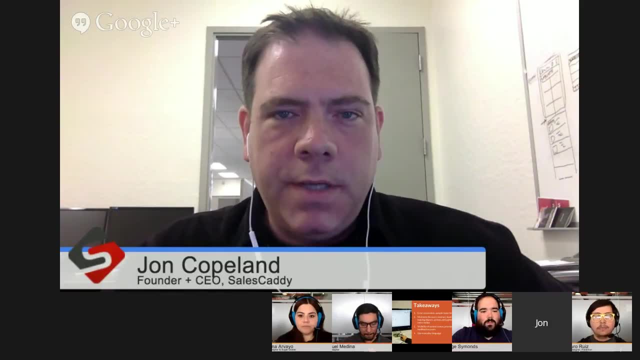 anything we can help you with right now. Actually, guys, this is great. What I really appreciate from your efforts and from what you provided today is you've helped us to really prioritize something that we just haven't been able to get from our key administrative users. 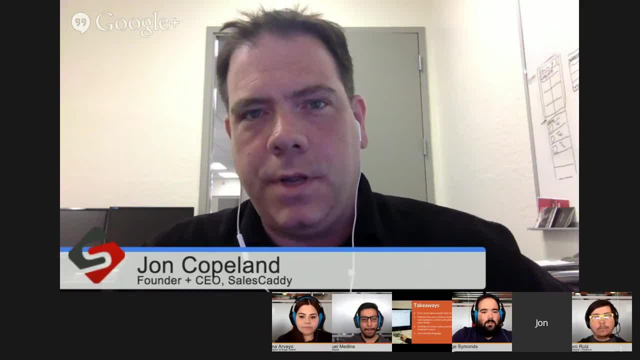 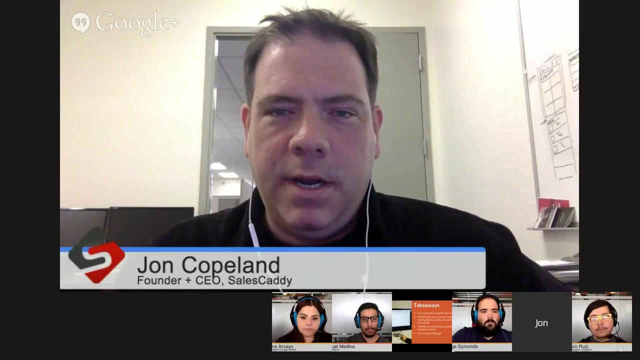 And just as a reminder to everybody who's watching, this is the console. This is what the business owners inside a corporation use to share, to watch utilization and to help administer all of the field-based users. This is an enterprise system, so that's a little context. 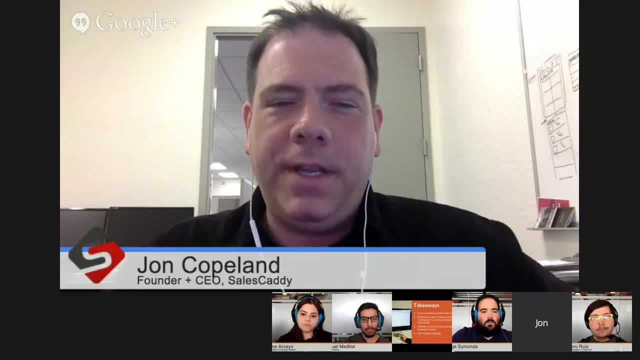 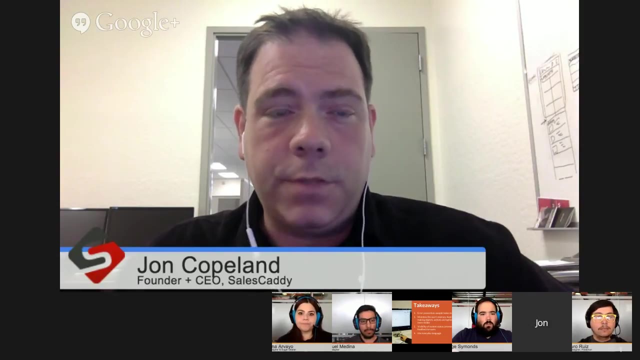 These are all points that are painfully needed and clearly needed. The way you've presented it, though, is really helpful. It's really helpful because you've prioritized it. You've explained a lot of the real reasons for the need to improve user experience in. 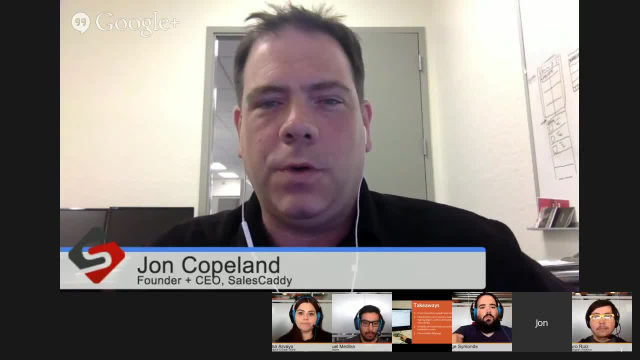 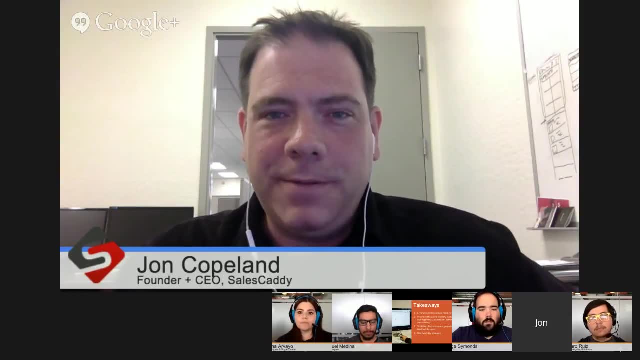 these areas, And what I really appreciate is you've given us a short top four things to attack, and so we can get right at it. So that's my first reaction. Great, Do you see this as coming alive in the next design iteration? 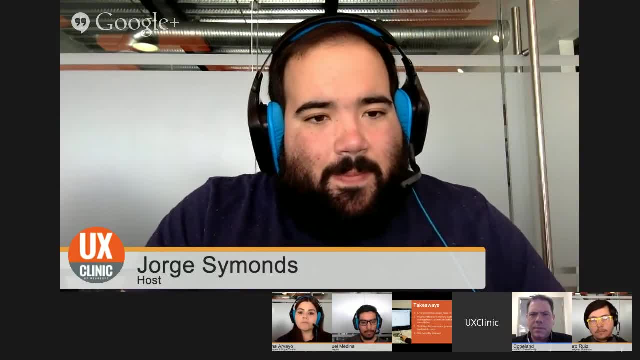 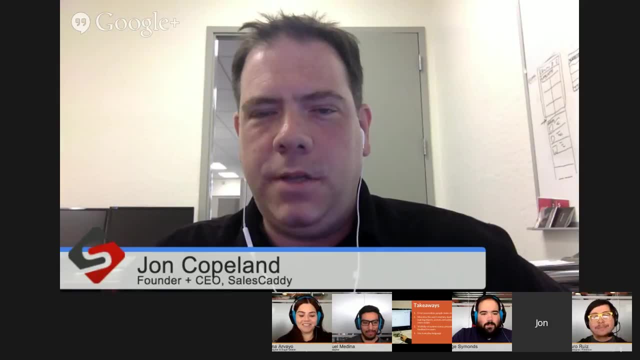 Do you think this is something you guys are going to use? Absolutely. I have a list of tickets a mile long. product requests changes to the UI. But we wanted to get some professional advice from UX Clinic and NearSoft before we just started diving in fixing random things that caught our eye. 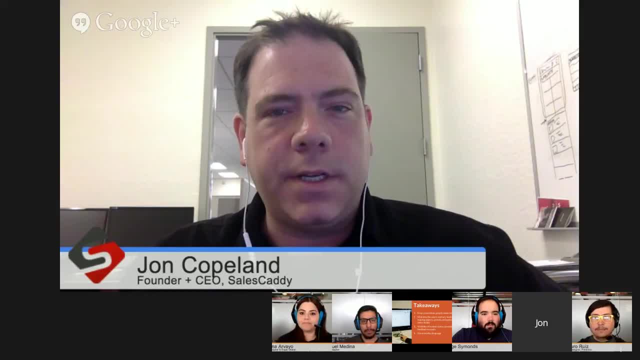 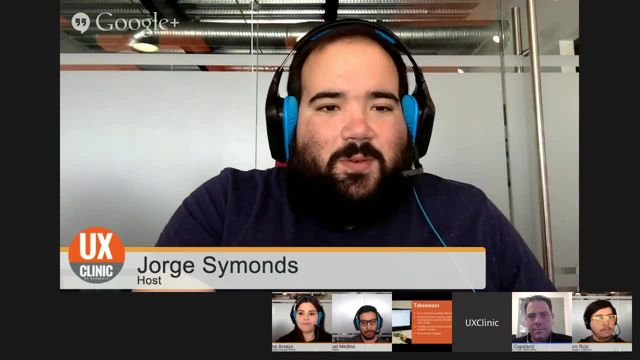 This gives us a runway, And so we'll put this into the next version, absolutely. Thank you so much, Guys. any last questions you want to ask John or John, any last questions you want to ask the design team? Or should I just say goodbye? 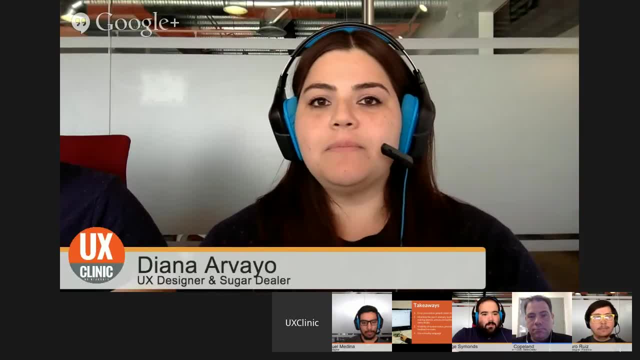 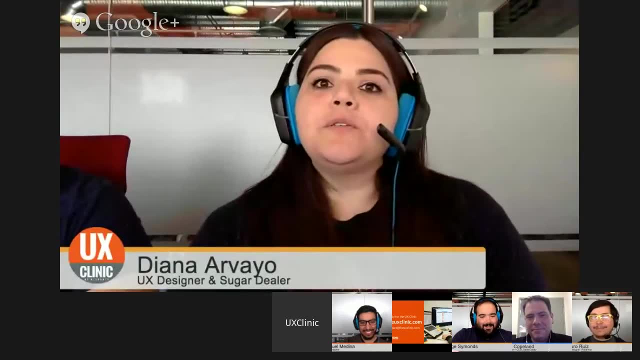 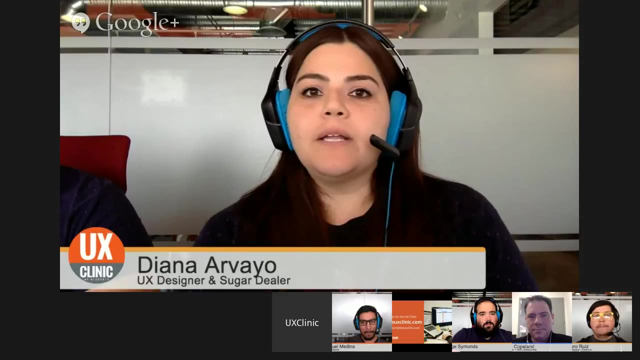 Well, I just want to thank to all my teammates here- and Marisol, we miss you, Just kidding, Yeah, Yeah. I just want to thank to all the participants, the four users that we had the interviews with them. Their feedback was super professional. 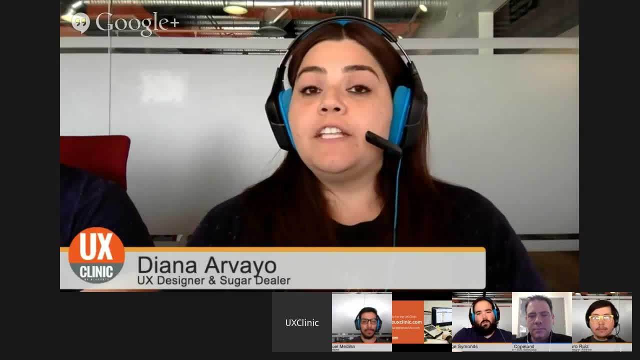 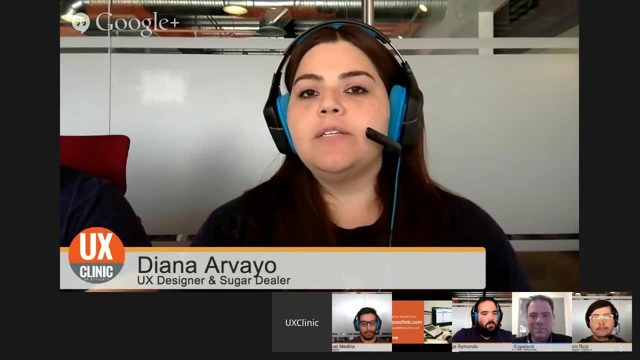 They helped us a lot also with the findings, And that's it. I just want to thank to John To the opportunity to be here in the UX Clinic. it was amazing to work with the Sales Caddy, So thank you so much. 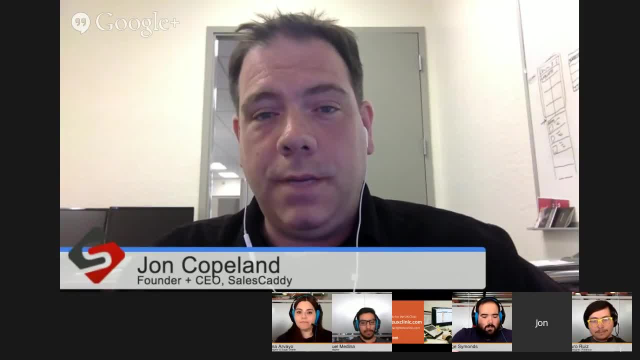 Well, thank you. It's a real pleasure to work with the NearSoft team and be a part of UX Clinic Again. I also want to thank our users Again. this is enterprise software and getting usability testing from them is really quite a feat. 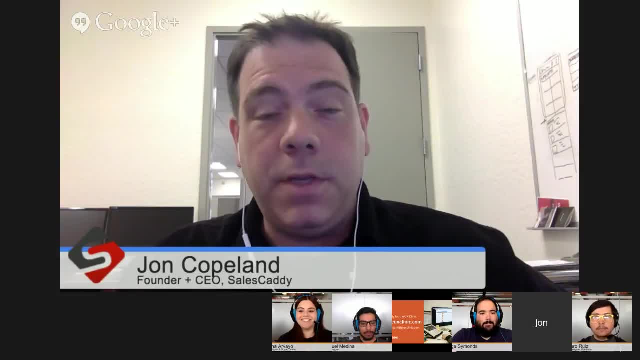 I'm amazed that we got as many testers as we did, and very grateful for the people who took time out of their busy day- Of course, your team included, but also our customers- to come together and provide this really valuable feedback and something that's actionable, something that's going to make. 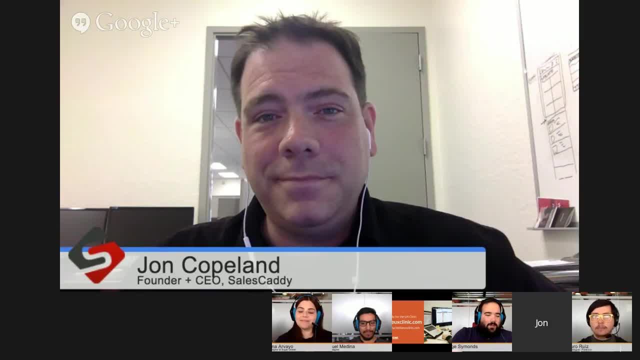 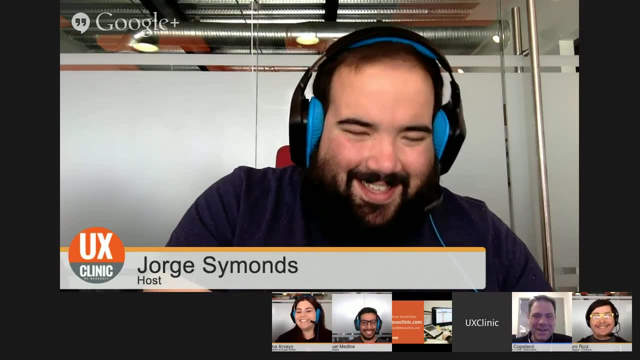 a difference with our product. So we're going to have to sign you up on the next chapter of the UX Clinic to see how the changes went and everything went down. I think that would be great. I'll take as much free advice as I can get. 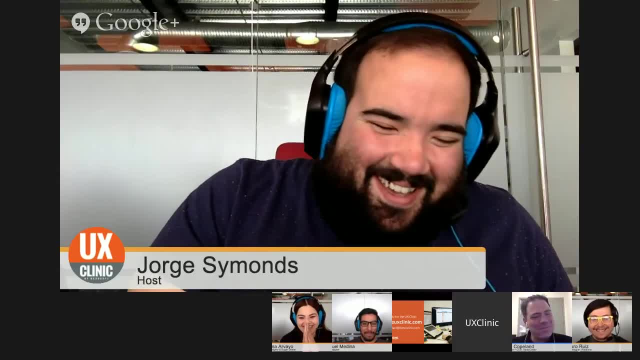 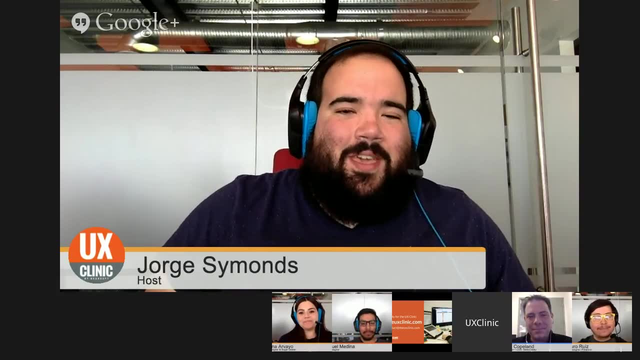 We're going to quote you on that. No, I'm kidding. So, guys, that's our show for today. It was great having you on board, John, and the whole design team. I want to thank the audience, too, who was here with us, and especially Vani. 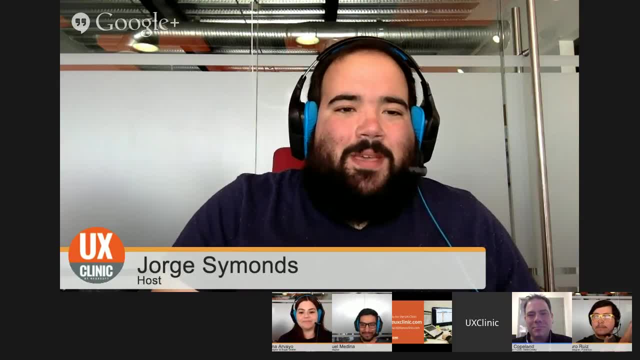 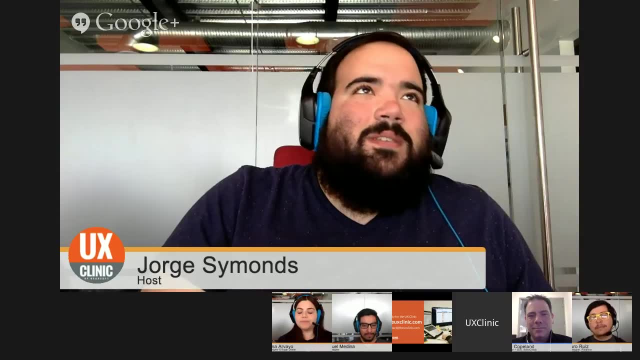 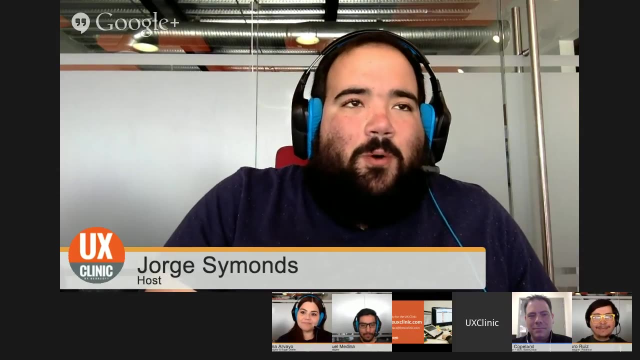 Vani is always off camera, but he's always making everything happen, so claps to him. I'd just like to remind you that making a delightful, user-centered world is all about making money. to be honest, This feature that you can change on your product will probably make you more and more money. 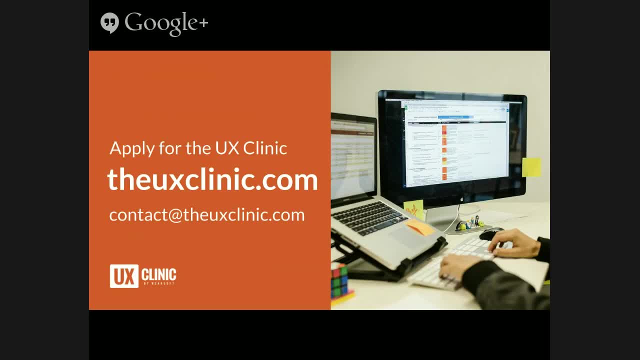 so we're in the business of making great companies. It's great software for great users and the end money. so send us a request at contact at theUXCliniccom or through theUXCliniccom website and we'll be happy to feature you.